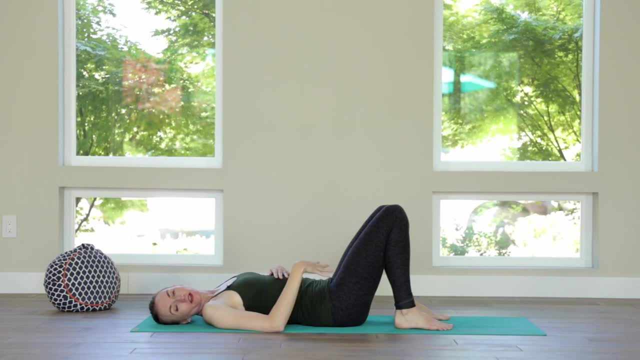 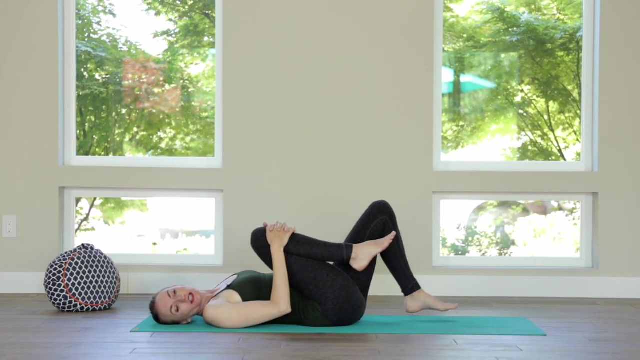 Does one side of the low back hip sacrum feel weightier And just breathe And then gently pull the right knee into the chest And you're just going to let this left leg go long and give it a little bit of bouncing. You can hear I cracked right away, Just kind of. 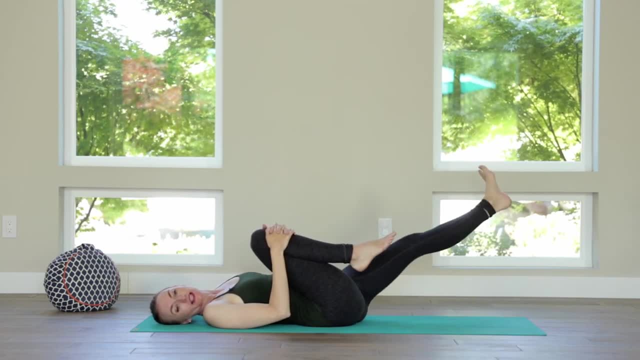 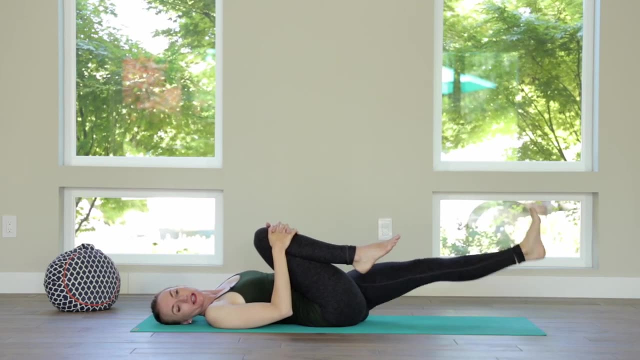 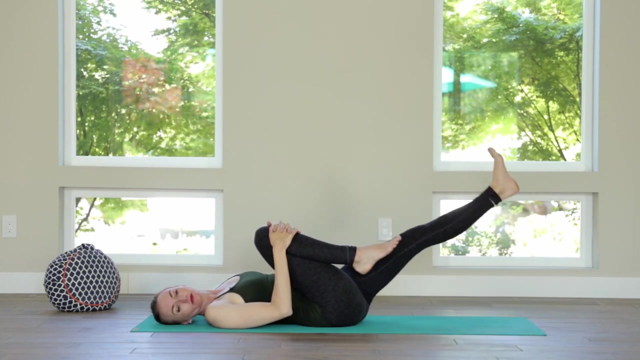 let it bounce up and down. You can take it a little bit out to the side If you want, not too much, a little bit across the body, but not too much. Just let it keep bouncing. A little gentle abdominal engagement here. 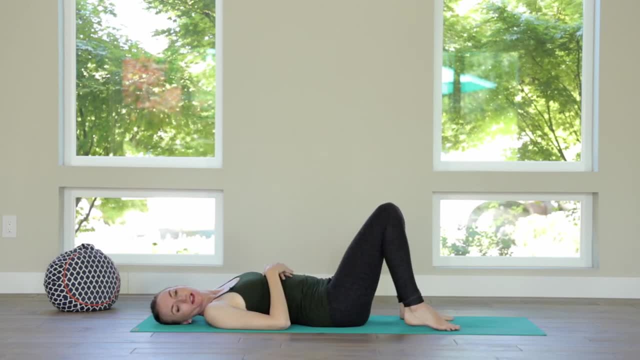 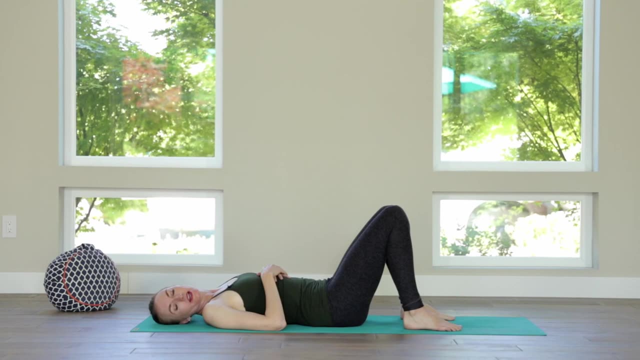 All right, that's good. And then take both soles of feet to the floor again, Close your eyes, Let your low back really settle and press down into the mat And notice if anything's shifted or changed. We'll do the same thing on the left, So pulling the left knee into the chest, This time the right leg. 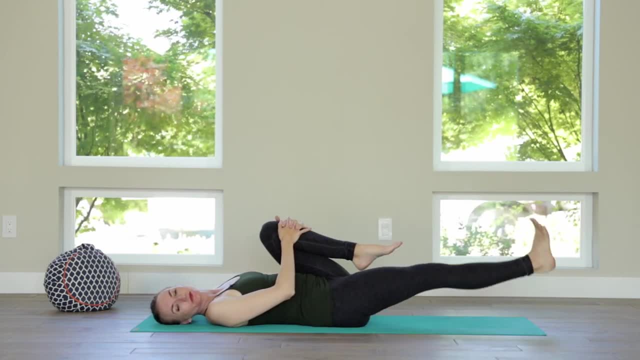 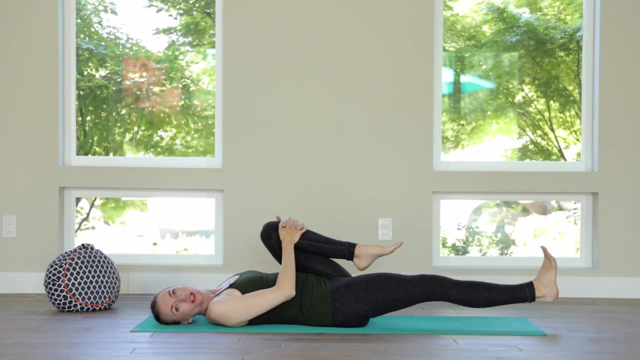 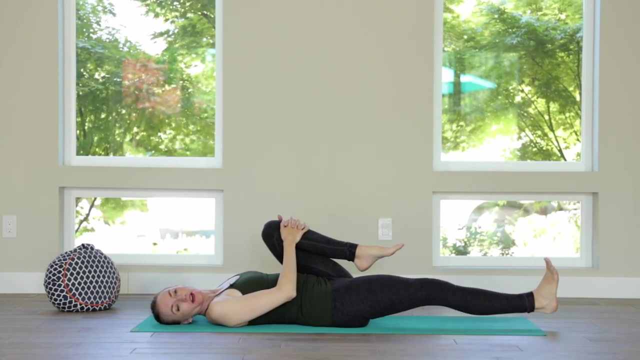 extends and just does some of those bounces. This should not be like huge violent bouncing that strains your low back. You can keep it really small. We're just trying to kind of work out any kinks in sacrum SI joint area before we continue the rest of class. 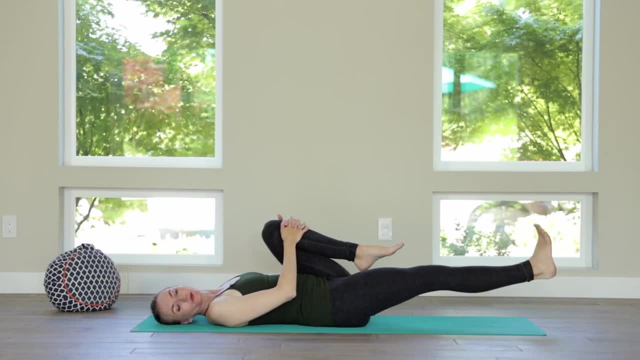 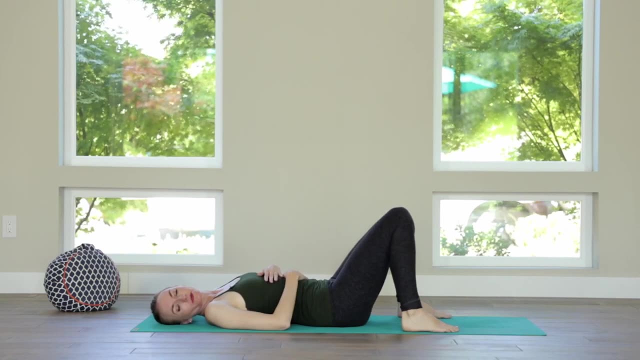 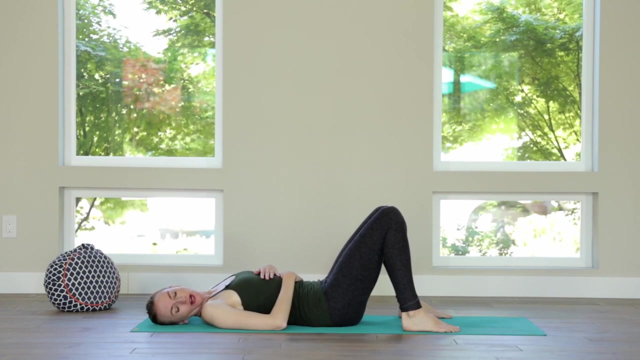 All right, and then both soles of feet on the floor and just observe. Maybe let your low back dip deeper into the ground. Take your shoulders a little bit more towards the top of your sticky mat, See if there's any length you found. 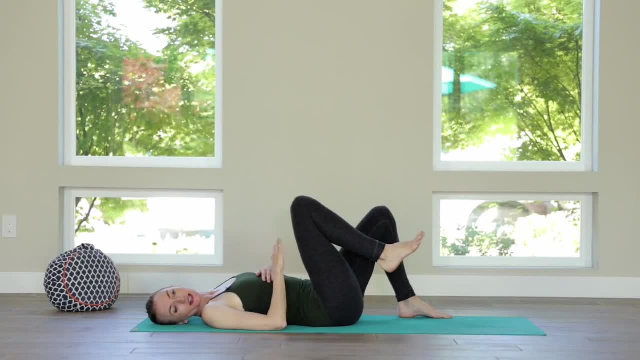 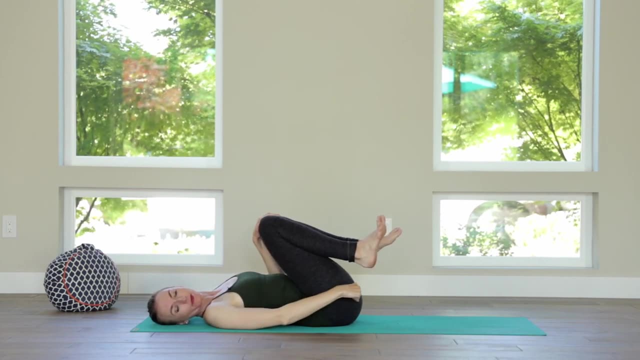 And coming into a standing position, Apanasana. So you're just going to hold your kneecaps. Visualize your two sitting bones like eyeballs that want to peer down towards your sticky mat. So keeping that in your mind's eye. 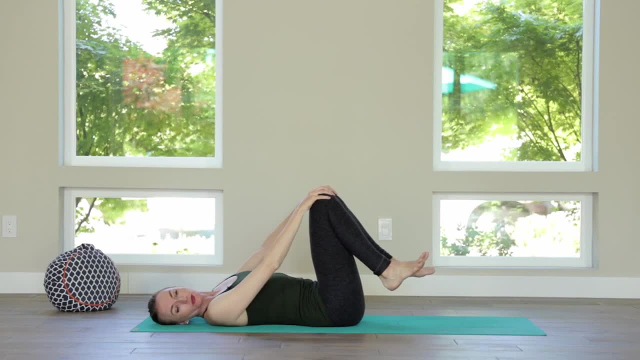 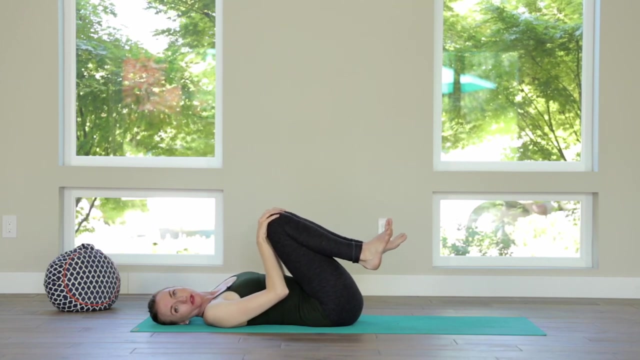 On the inhale. straighten your elbows, Let the kneecaps move away from you. Think of crushing a penny with your tailbones. Your tailbone also yearns forward. Those eyeballs of your sits bones yearn forward And keep that Exhale. bend the elbows, bringing the knees back. 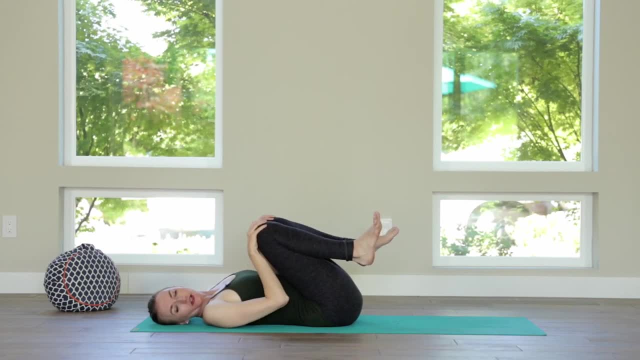 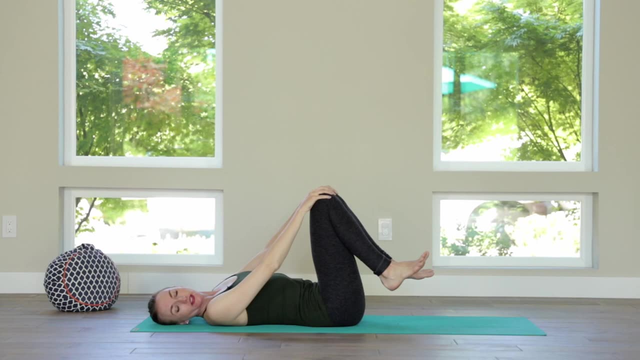 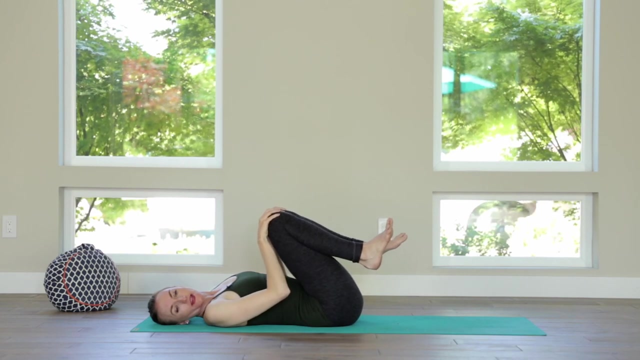 in. So again, this is subtle Breathing in Eyeballs of the sits bones peering down towards your sticky mat, And they keep peering down even as you bend the elbows and the knees. come back in. Just do this two more times on your own. 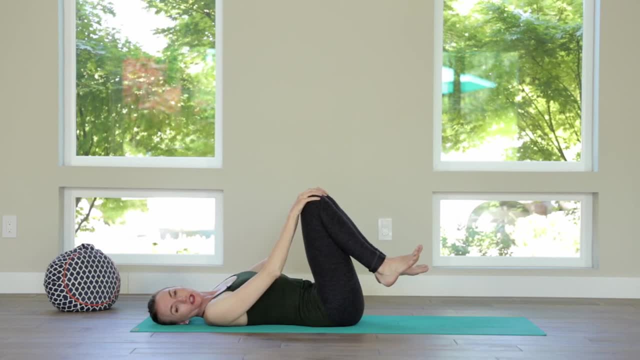 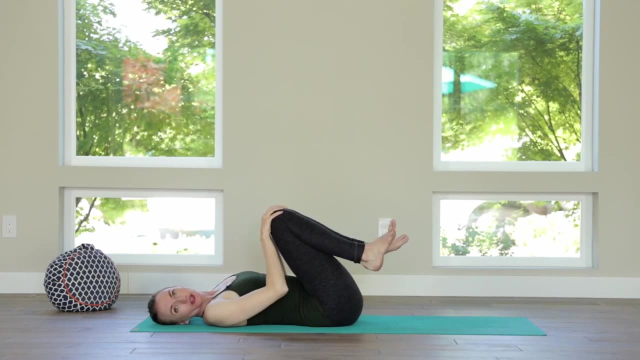 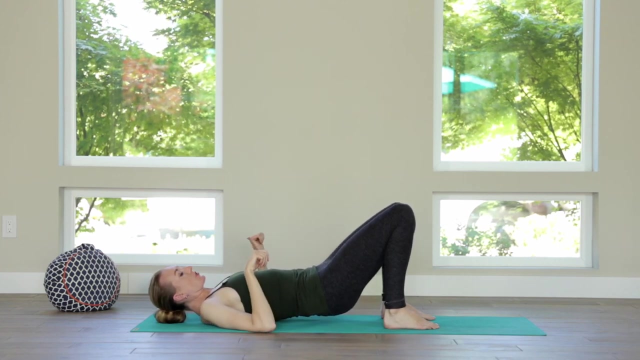 When we're working with low back pain or wanting to stretch this area, it's the most gentle therapeutic movements that really have the most effect. Nice, Take the soles of the feet to the floor, Lift your hips up And take the hips two or three inches over to the left. 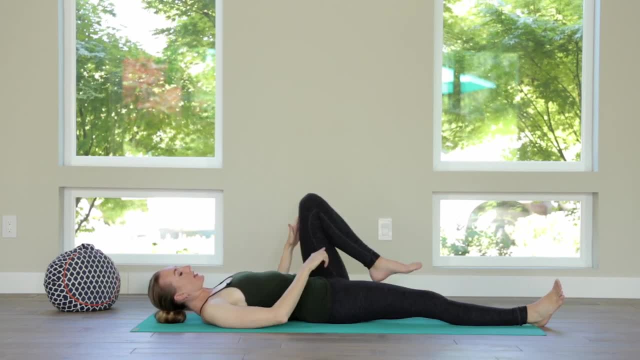 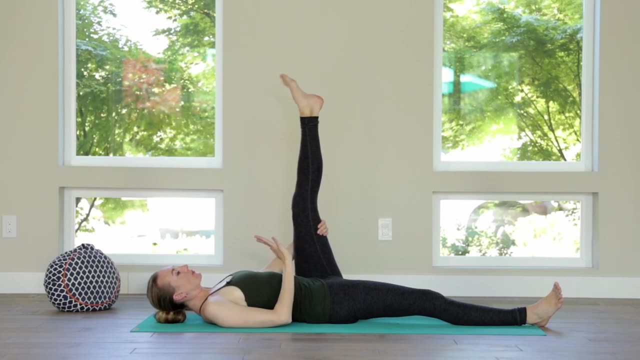 Allow your right leg to straighten Left knee. you're going to pull it into the chest And then straighten the leg, Doesn't matter how much. This isn't about a stretch or anything like that. You're just going to let that left leg drift over to the right. 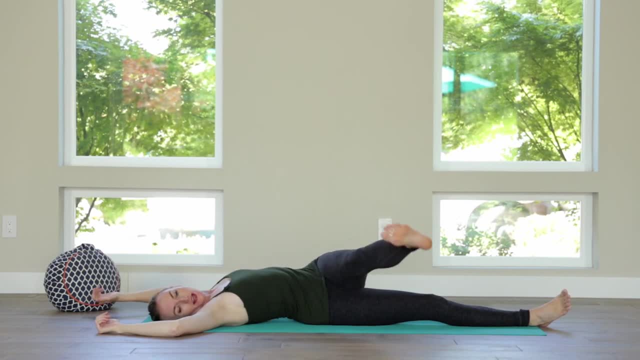 It's okay if this hip, the left hip, comes up off the mat And then come back up And over to the left Again. let's think of this as more as like we're finding more space in the sacrum, on the left side of the sacrum, Then we're not trying to get an IT band stretch or a. 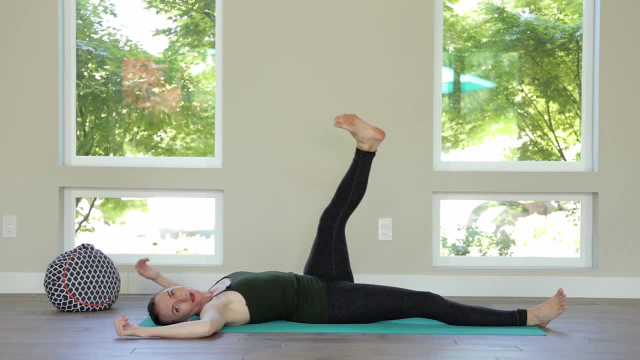 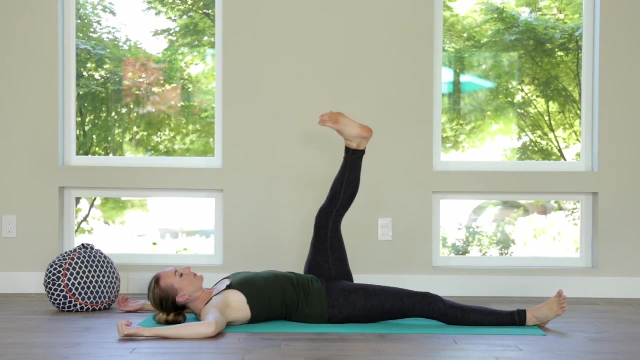 hamstring stretch or anything like that. You're just kind of rocking here And then just look straight up towards the ceiling: Good, Good, Good, Good, Good, Good. One or two more Again. this isn't about flexibility. Hopefully you're starting to feel. maybe the left side of 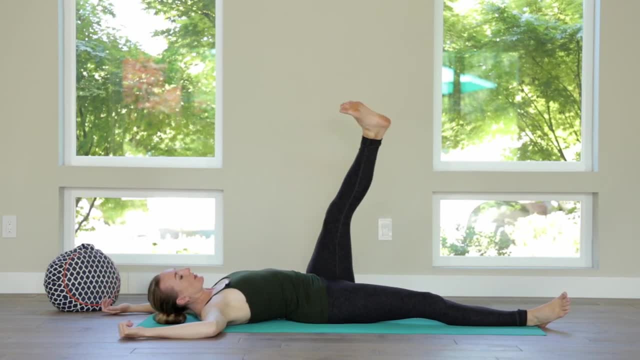 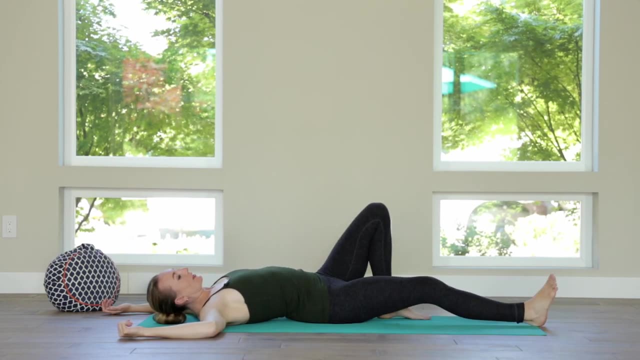 your low back sacrum, open up, Good, Take the soles of the feet to the floor, Bring your hips back to center And then really pause here and notice the difference between the left and the right. Okay, Good job. If you felt the difference between the two sides- left side of the low back sacrum and hip- how it feels. 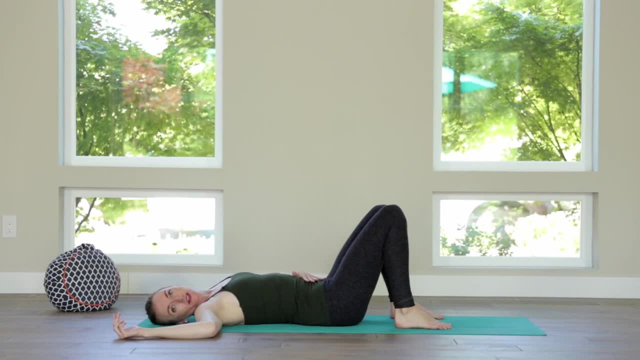 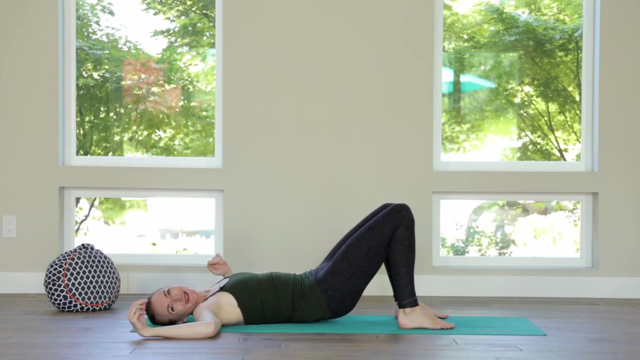 connected to the mat as compared to the right. Good Eyes closed, deep breaths. Lift the hips up as you press into the soles of the feet. take the hips two or three inches to the right, let the left leg go long and the 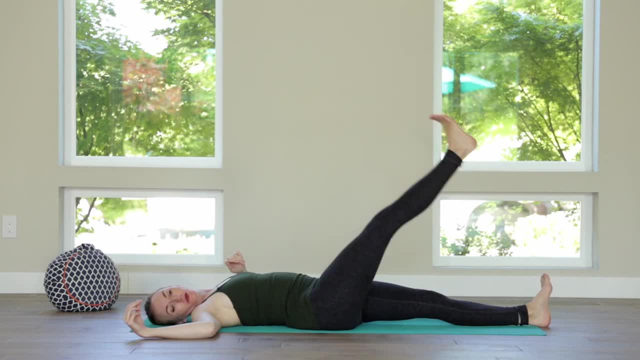 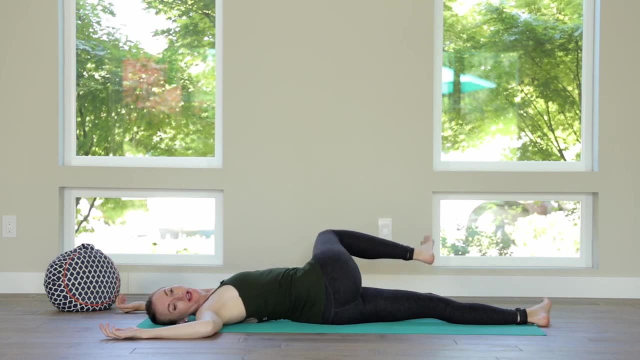 up just as much as to your ability. If you know the leg's way down here, you can always keep the knee bent to do this exercise right, And we're just taking the knee over and back up, over and back up. And, of course, if you had the leg straight on the first side, 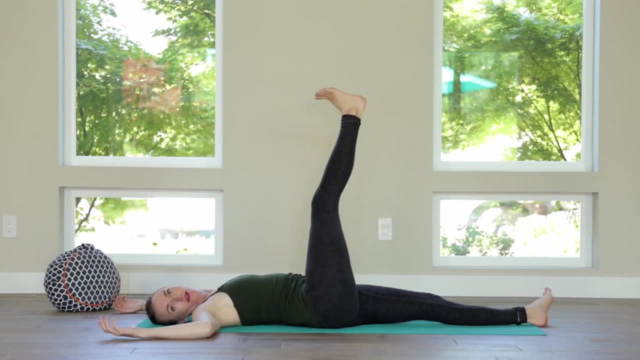 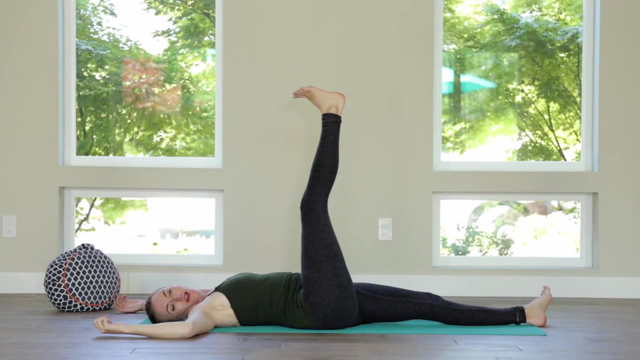 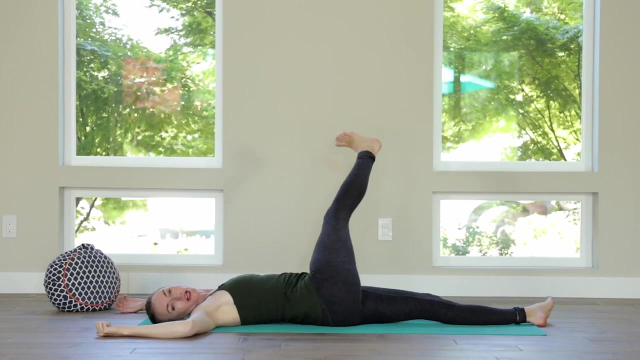 right straight over. this is more intense back up. It's this area that we're focused on bringing in some gentle movement and mobility. Forget about a hamstring stretch, Forget about IT band stretch. It's all about the low back right now. 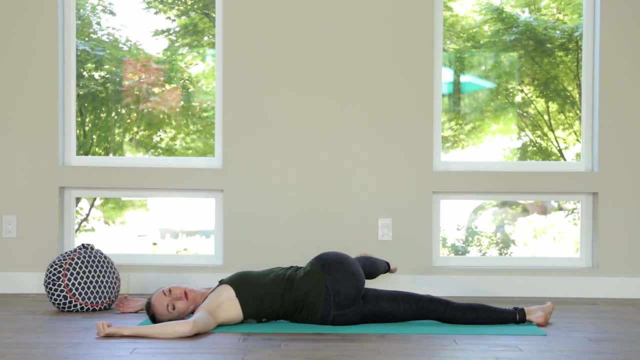 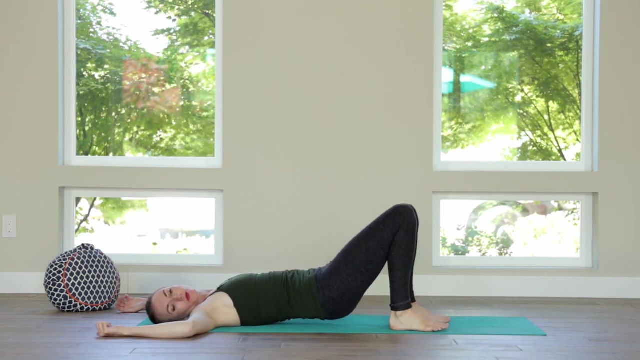 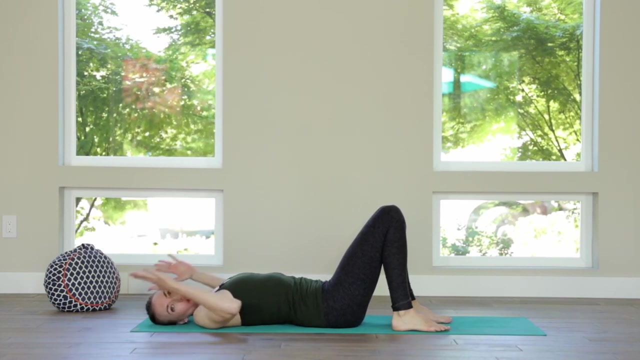 Good, And when you're ready, slows of the feet down, lift the hips, bring the hips back to center And let's just do a couple bridges here So you can just keep your arms in a goalpost shape. or you can do like little robot arms, like I'm showing here, the biceps pressing down. 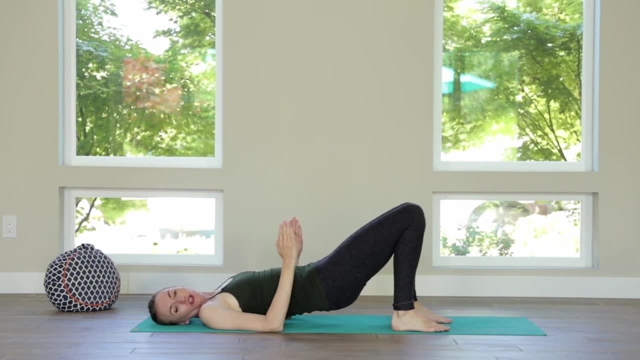 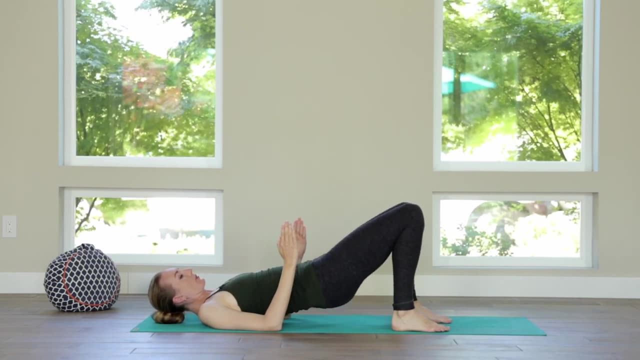 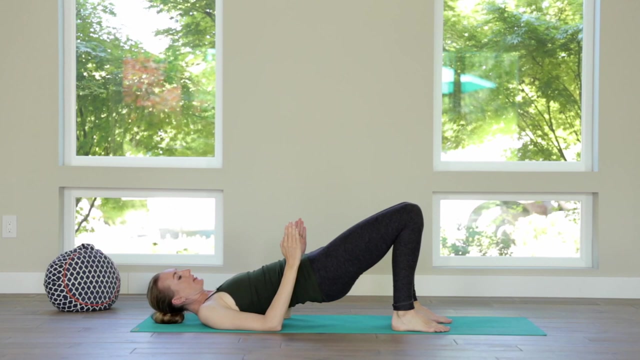 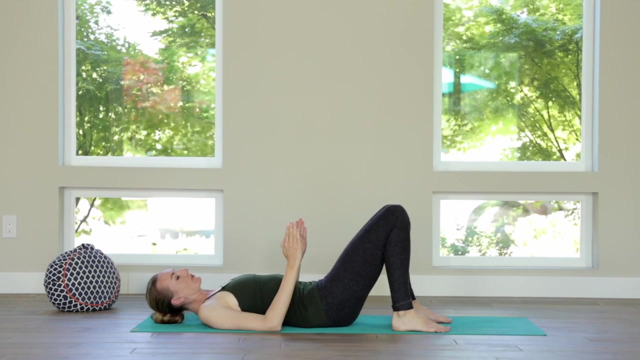 fingertips up And then you're ready to go. I'm just going to lift into your bridge and look straight at the ceiling. Just a couple. Think of your tailbone lengthening towards your knees and make these slow Good, And then take your feet a little bit wider apart. 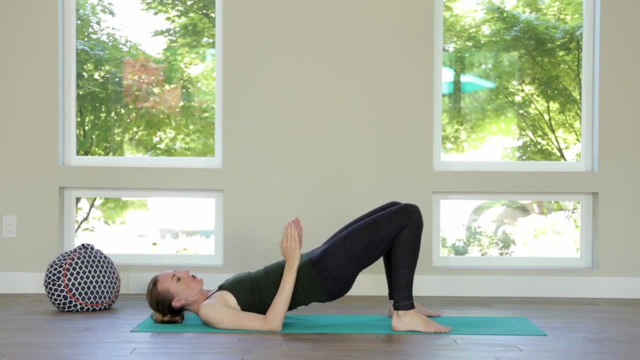 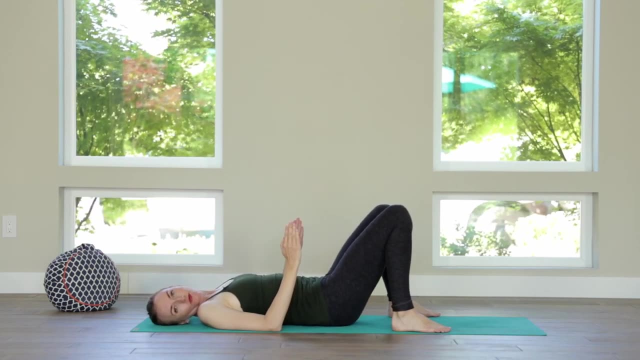 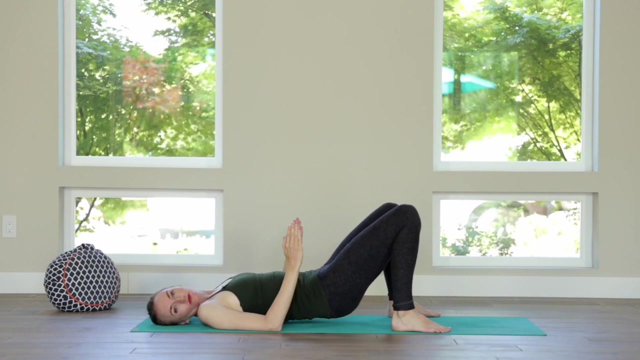 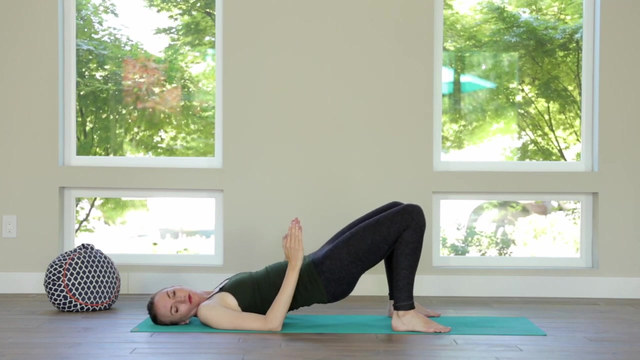 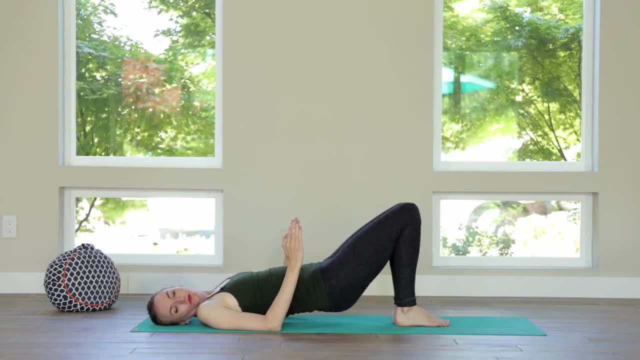 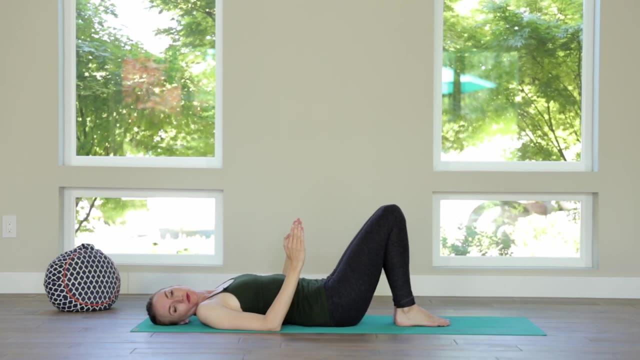 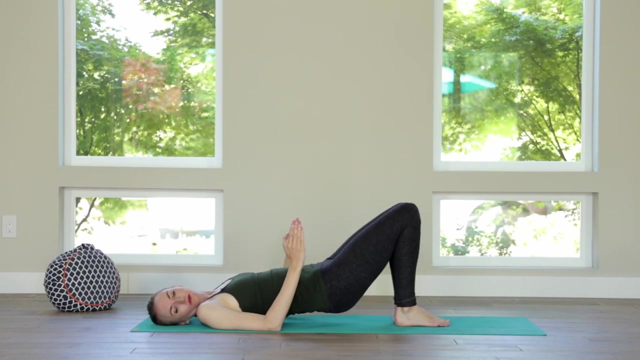 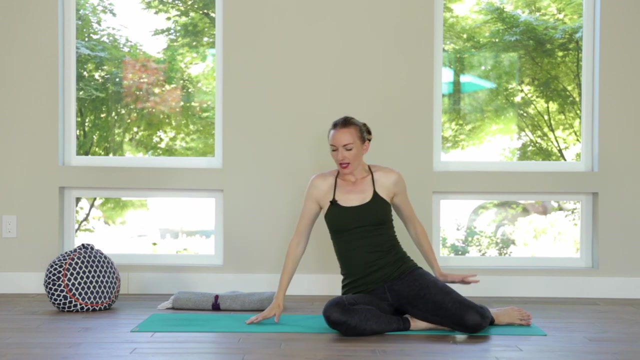 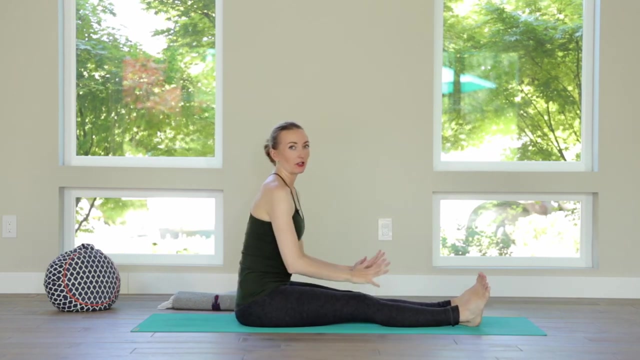 Just five: Inhale to lift, Exhale to lower. When you're done, you can pull the knees into the chest, Roll to the right side, gently press yourself up and just sit with your legs long in front of you or, if that's uncomfortable, 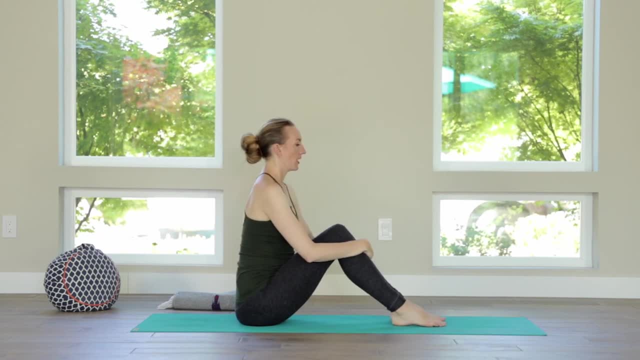 you can just sit with the soles of the feet on the ground and just notice how your low back feels again. it may not feel like this crazy stretch per se, but maybe it feels a little bit more wide and open, relaxed. and we'll close with Janu Sirsasana. 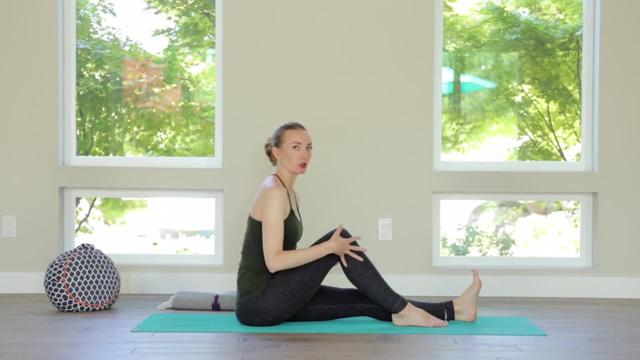 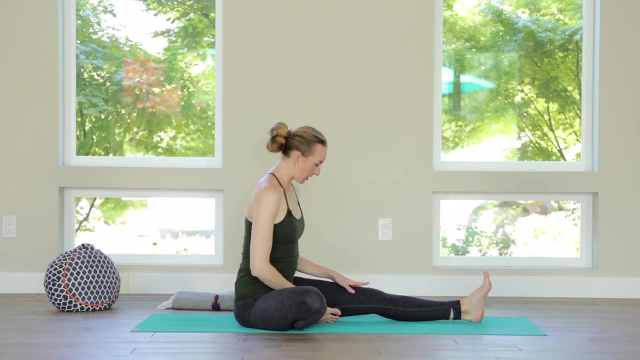 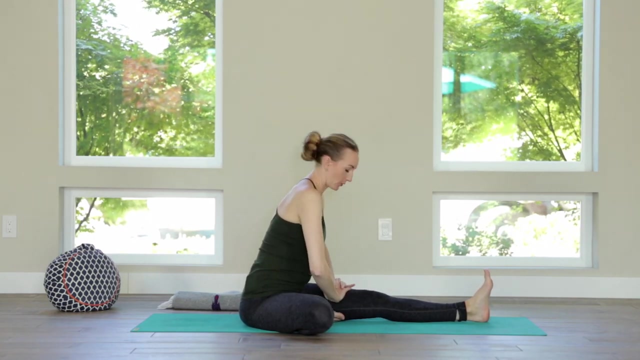 which is more of a traditional stretch, but I think is so much more effective after we've stabilized the low back in this way. so right foot into the left inner groin and just for our focus today we won't even take the arms up, we'll just press down into the left thigh. 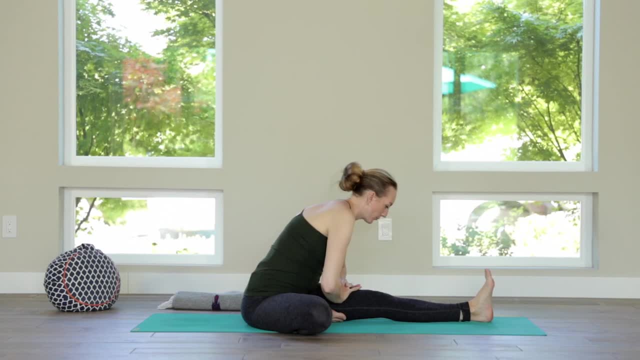 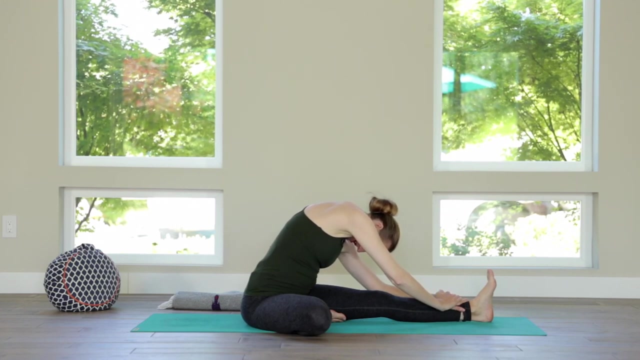 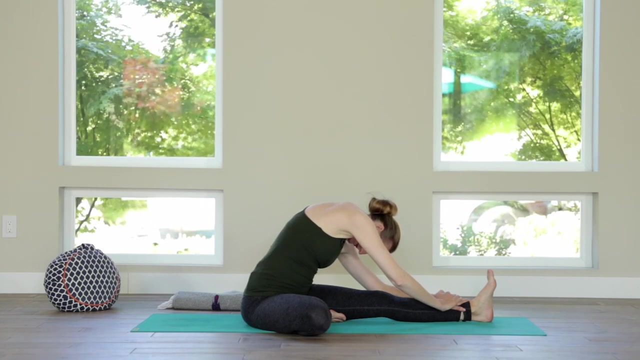 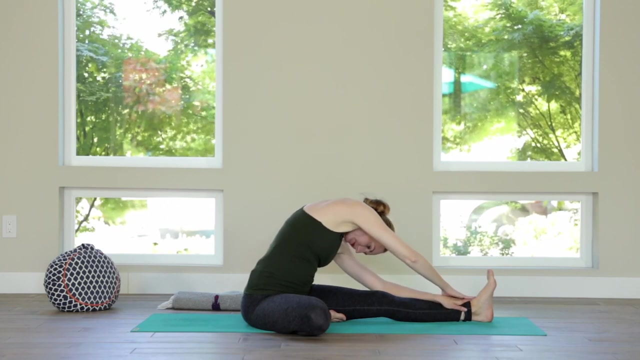 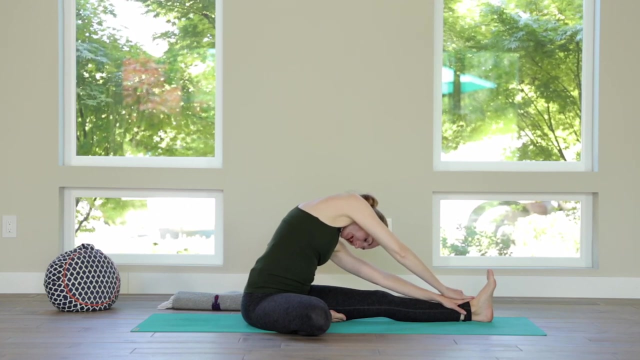 lift the heart and then exhale. fold forward, you can hold, you can keep the hands right here, hold anywhere on the thigh, shin or foot and just take five slow, deep breaths. lean a little bit over to the left and notice if that opens up a stretch in a different way. 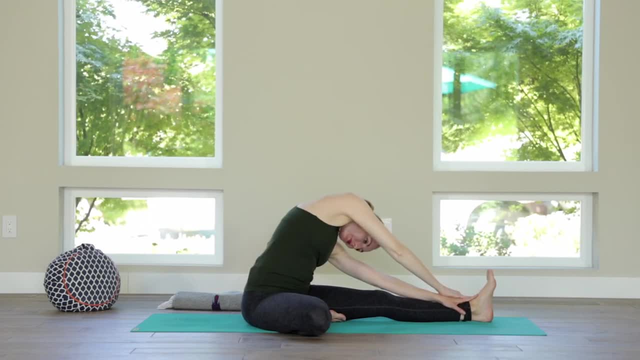 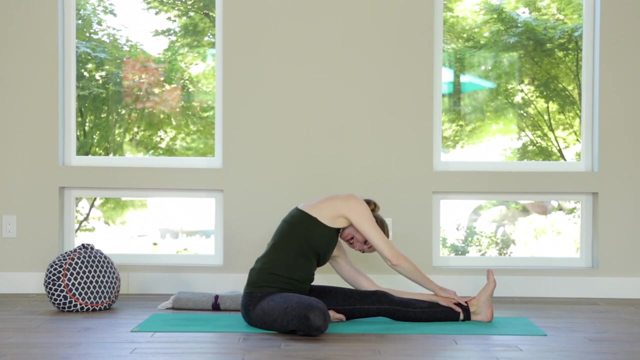 along the right side of the low back. for you it's kind of like your weight and your torso sort of fall left. we're not reaching for the foot, you're trying to feel a hamstring stretch or anything like that. just keep the hips heavy and the head heavy. 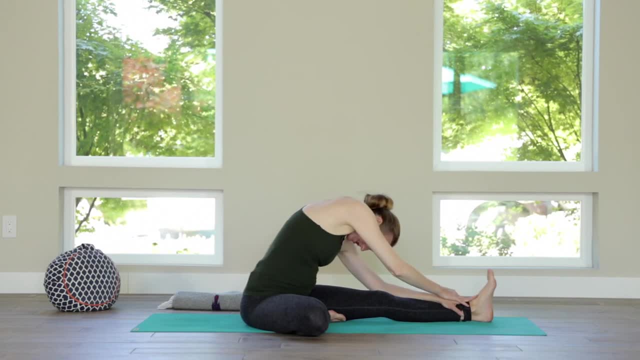 and it's okay for the torso to round, and then if you're feeling a little bit more comfortable with that stretch, just let it go, and let it go for the rest of your day, take the weight of the torso over to the right, and this if there's anything. 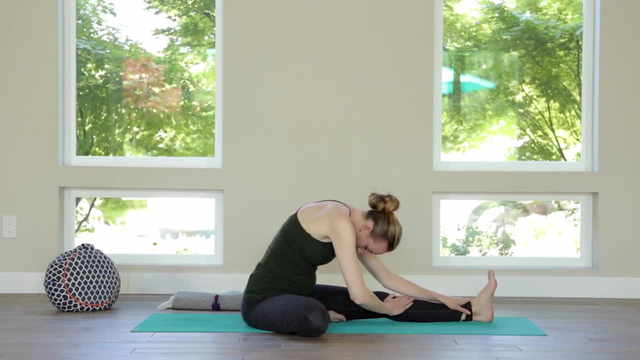 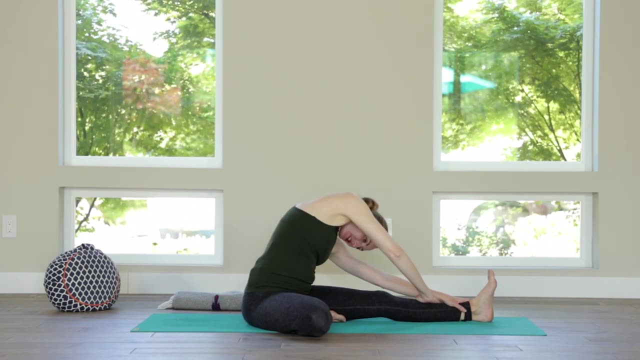 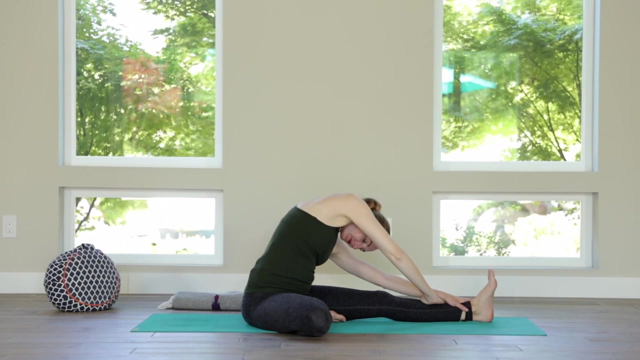 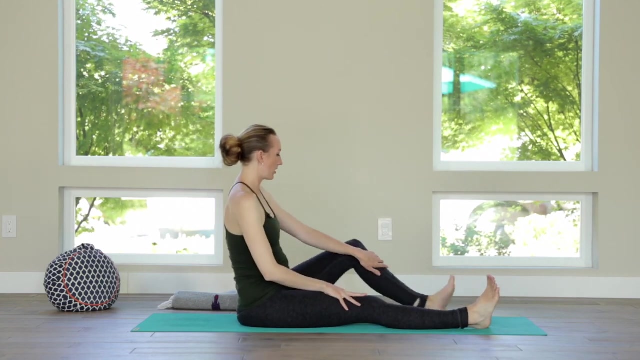 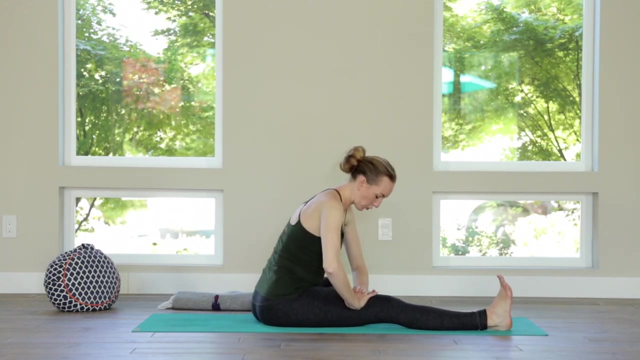 interesting there, maybe back over to the left. oh, it's more interesting to me. if you do feel sensation, really send your breath into that area of the low back and then walk your hands up and just switch the legs, so right leg long, left sole of foot into the groin, interlace the hands, press the right thigh. 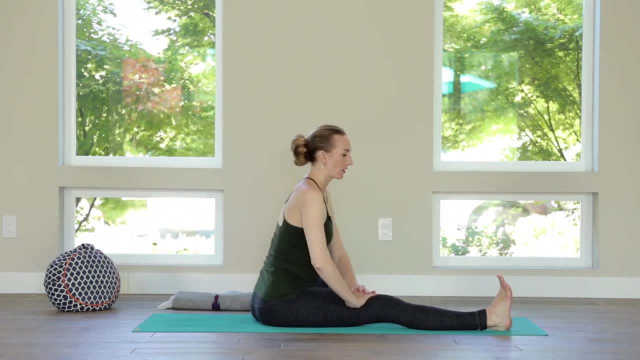 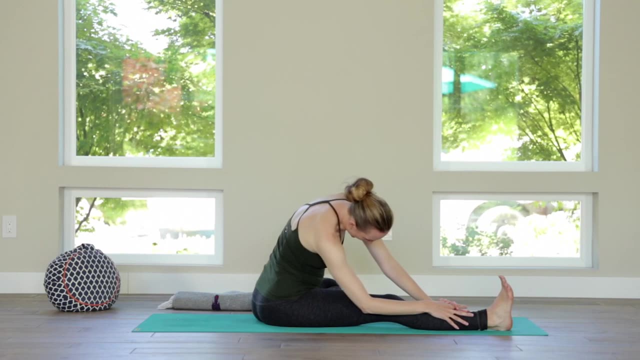 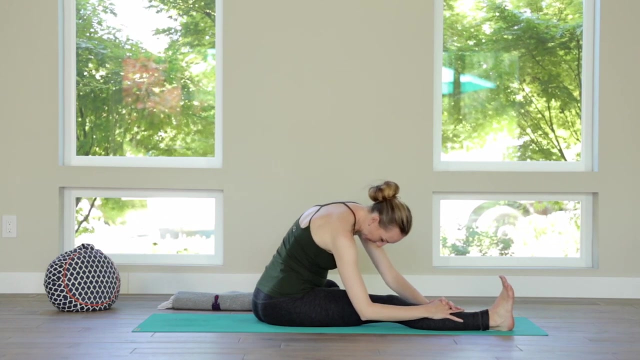 down. you then lift the heart and exhale fold again. we don't care about a hamstring stretch so much, but it is great to keep this right foot really flexed and powerful and then chin into chest head heavy like a bowling ball. you can hold here for a few seconds and then lift the heart and exhale fold and then. 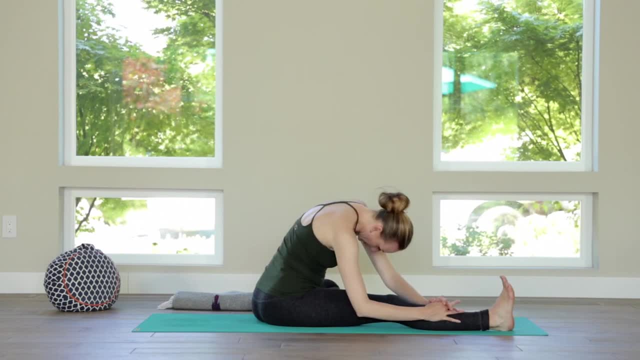 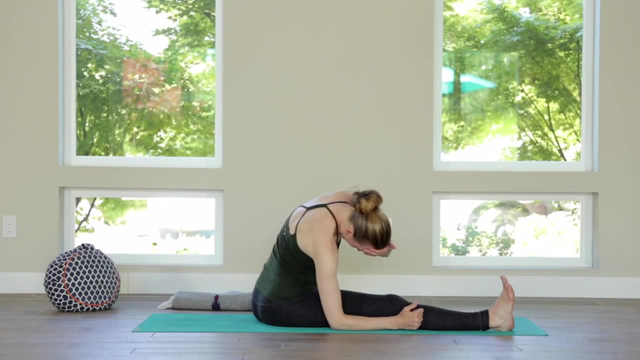 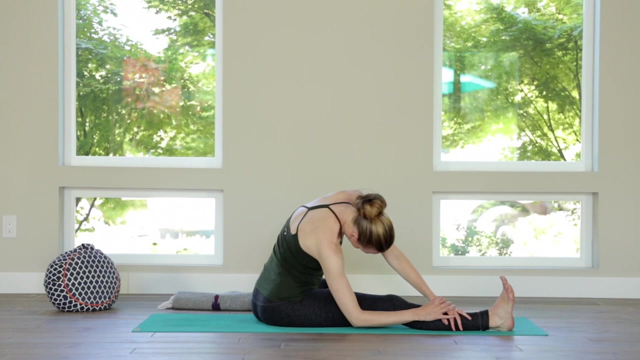 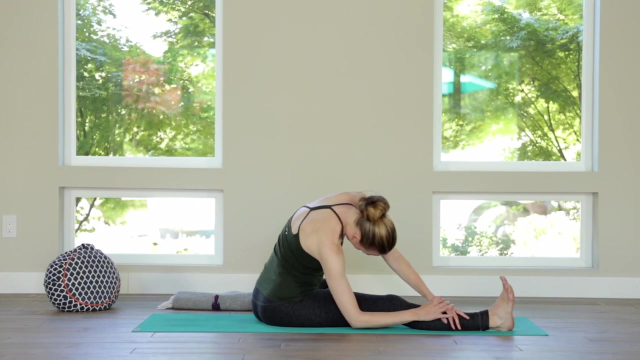 here for a couple breaths or right away. start kind of playing like I did on the first side, rocking and sending your body weight over to the right and looking for a stretch on the left side of the low back. take the body weight over to the left just to see what that feels like. if you 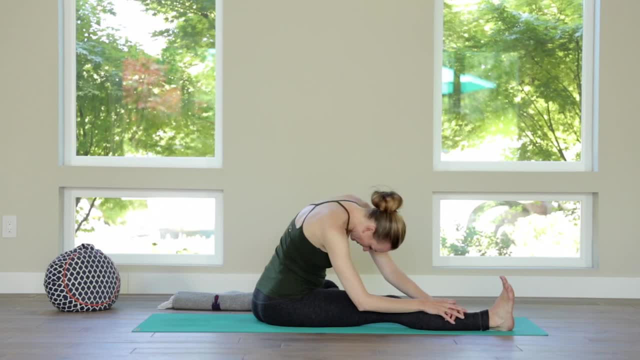 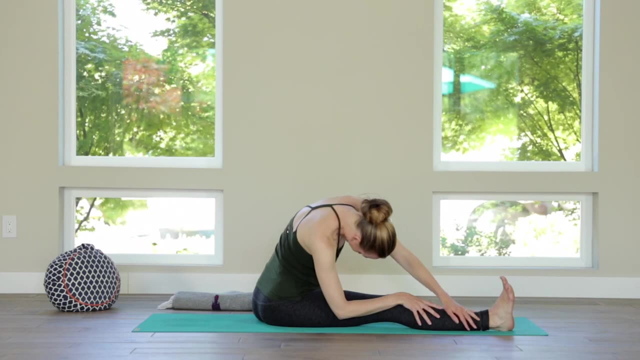 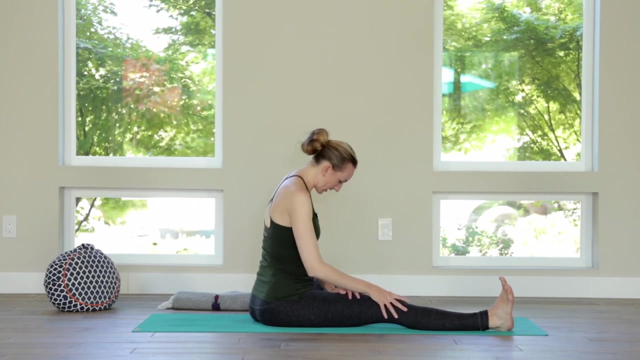 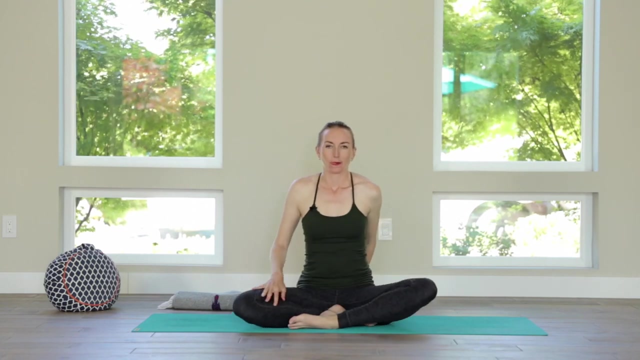 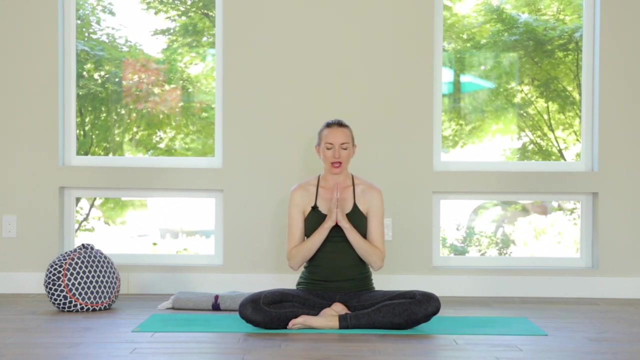 want two more breaths. you, you, you, you, you. you could walk yourself back up, come to a cross like a feat. bring the hands to prayer at heart center to close your practice. take a couple breaths here, breathing down into the low back, the hips, noticing if anything has shifted for you. feel more relaxed, please feel more relaxed. 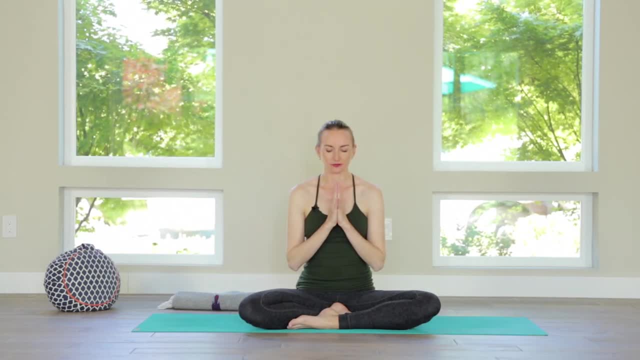 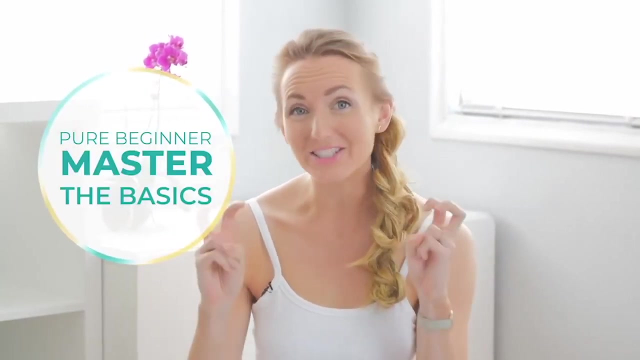 in that lighting too, though, and then we'll see you again soon on the road here to theouday light, usual��등 more space, and I'm sending you so much love from my heart to yours, Namaste. Hey, if you like this video, you are going to love my free, pure beginner. master the basics.